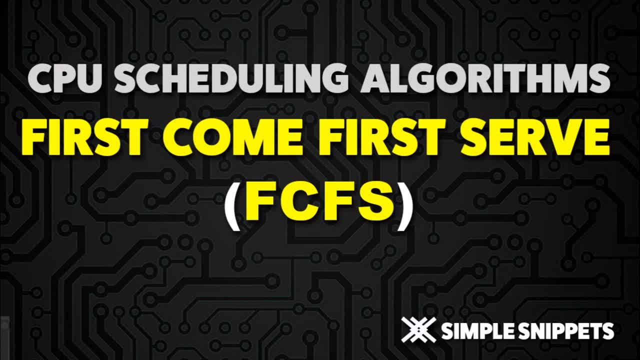 looking into the first come, first serve CPU scheduling algorithm, also known as FCFS. So basically, CPU scheduling algorithms define how a CPU will schedule and process different jobs and processes. So we won't be getting into a lot of theory, Let's straight away. 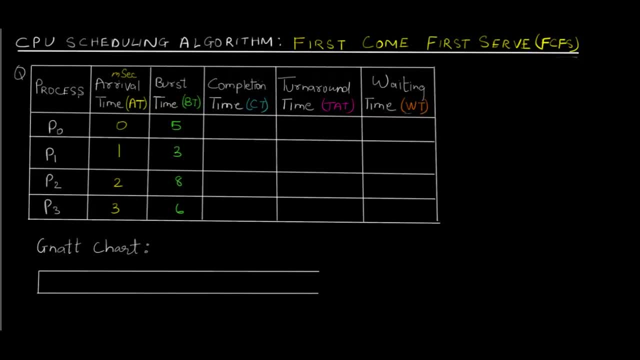 jump into the numerical. So, as you can see on the screen, we've been given a table with certain quantities. So let me just tell you what all details have been given the question We have been given with the processes. So we have four different processes: P0, P1, P2,. 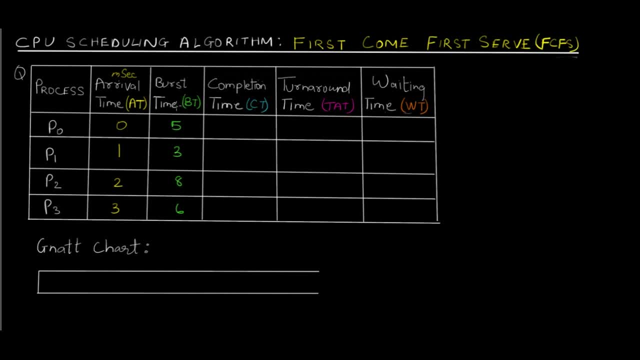 P3.. We've been given the arrival times of each of these processes and the burst time, So the arrival time is the time at which the process entered the queue. So for P0 it is 0, for P1 it is 1, and in this case the quantity or the value is in. 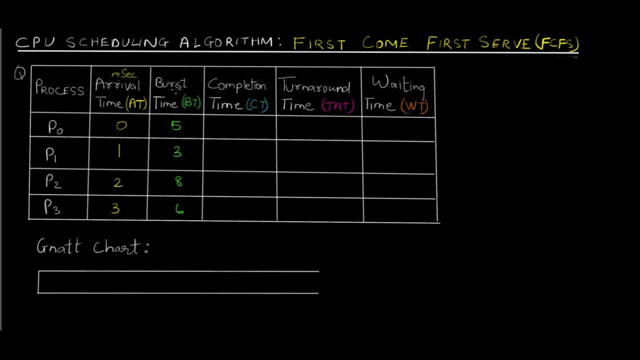 milliseconds. The unit of measure is milliseconds. Now the burst time is the time required by a particular process to complete itself. So when a CPU will start processing P0, it will require 5 milliseconds to complete that process. Now the remaining three quantities are supposed. 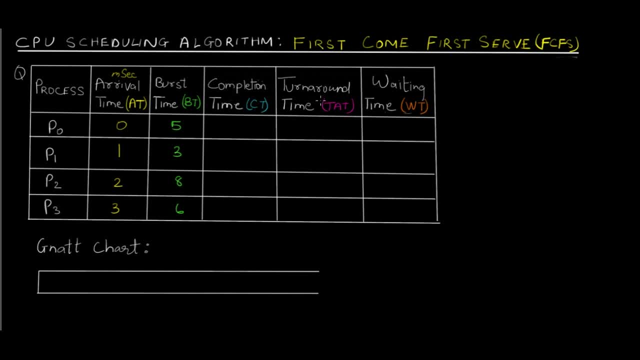 to be calculated by us. So we have to calculate completion time, turnaround time and waiting time. So, in short, completion time is the time when the process is finished by the CPU. The turnaround time is the time for which the process was inside the queue, So the 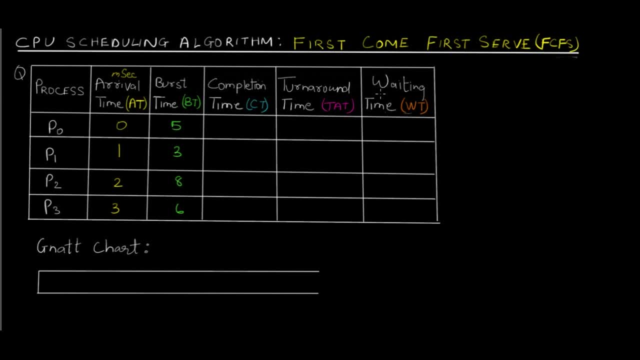 total time spent by a process inside the queue, and the waiting time is the time when the process was inside the queue but did not get CPU time or the CPU was processing some other process. So you'll understand that more clearly when we actually go ahead and 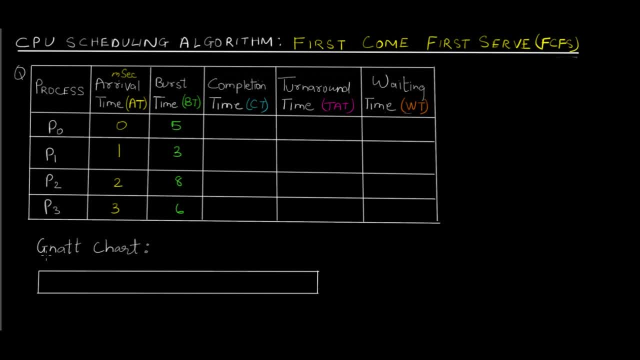 draw the GAN chart, and the GAN chart is sort of a timeline for when the process came into the queue and when the process completed itself. So since this is a first-come-first-serve algorithm, in this case the CPU is assigned to the process that comes first. 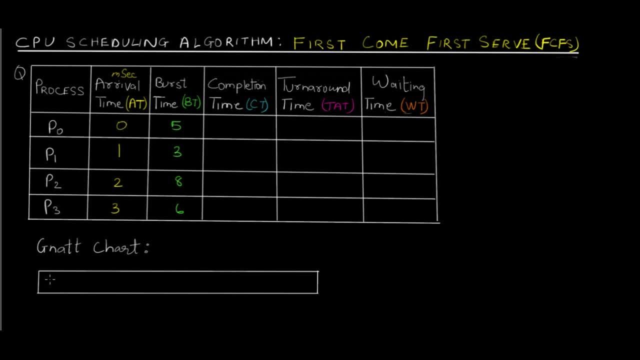 came in at time 0, so it came first, right. so we just have to write down p0 over here, and we know that it requires 5 milliseconds to complete. so if the timeline started at 0th second, we add plus 5 to that, and this is how p0 is going to look like on the GAN chart. 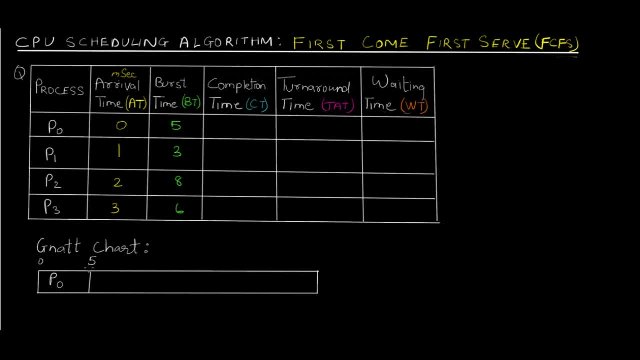 and the CPU is going to process p0 from 0 to 5 seconds. now if you see the arrival times of each of these processes, at time t equal to 0, only p0 had come inside the queue, but at time t equal to 5, by the time process p0 was completely processed by the CPU. all 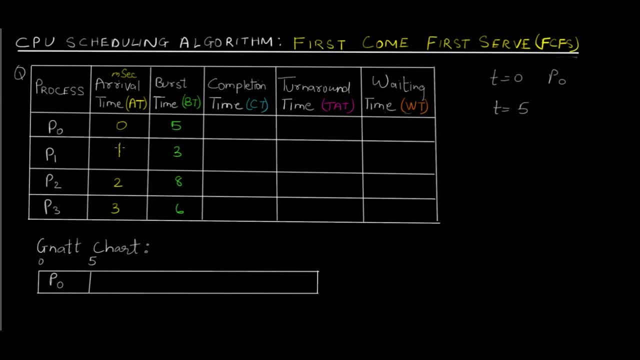 these other processes have come inside the queue right because the arrival times is less than 5, so at time t equal to 5. p1, p2 and p3 all came in this respective order, that is, p1 came first, then after that p2 and p3. but they all were waiting because p0 was still 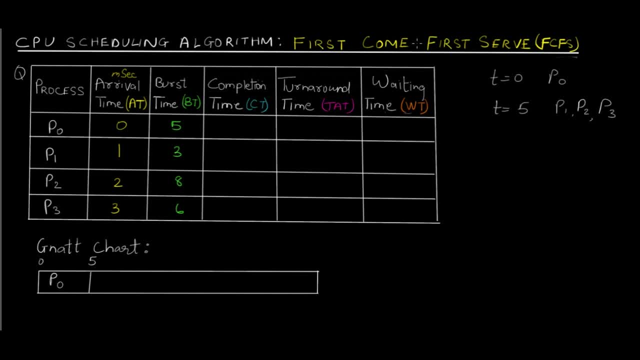 being processed till 5th second. now, since it is a FCFS scheduling algorithm, the process that came first and was waiting inside the queue will be processed next, after p0. so we know how it works. So we know, after p0, p1 came because the arrival time is 1, so we have to write p1 now. we know. 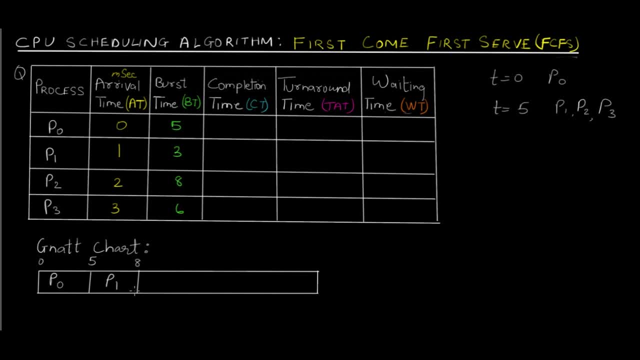 it requires 3 milliseconds. so 5 plus 3 is going to be 8 and this is how p1 is going to be finished by the CPU. after p1, we know p2 came into the queue at time equal to 2, so we will. 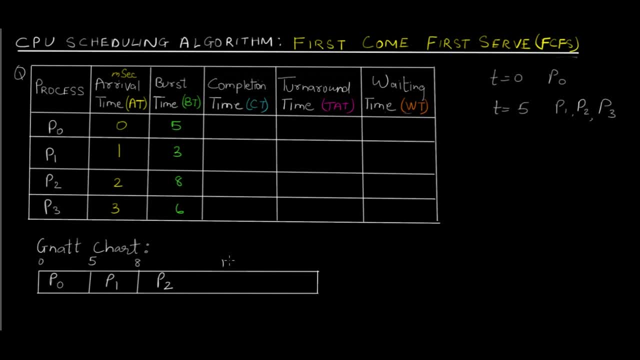 write p2, it requires 8 milliseconds, so 8 plus 8 is going to be 16, and this is when CPU will finish process p2. and last process is going to be p3. it requires 6 milliseconds according to the burst time, and it will finish processing at 16 plus 6, which is going to be the final. 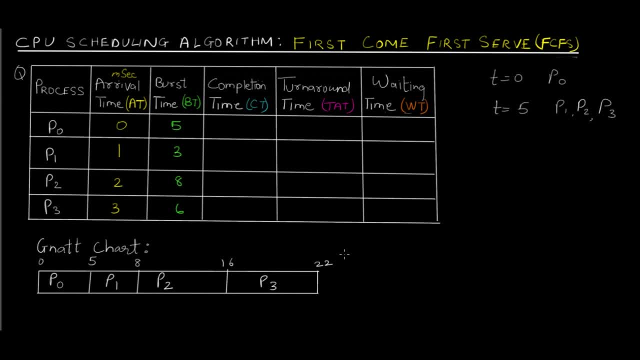 process. So this is the entire Gantt chart and using this Gantt chart we will now find the completion time. so completion time is the time at which the process was finished by the CPU. so for p0, we know it finished at 5th second, so I will just write it down as it is. for p1, the 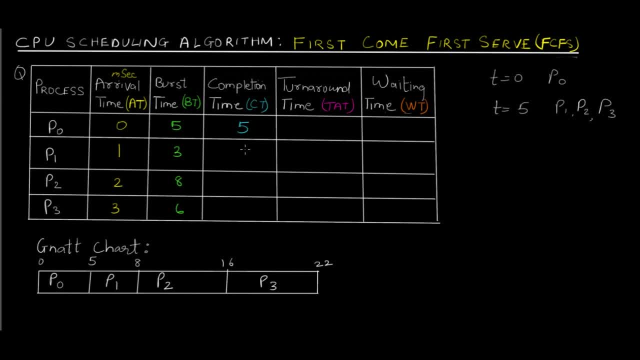 process. p1 finished actually at 8th second according to the Gantt chart. so we have to write down 8 over here. for p2 it is going to be 16 and for p3 it is going to be 22. so up until now it was pretty straight forward. we got all those values just by looking at. 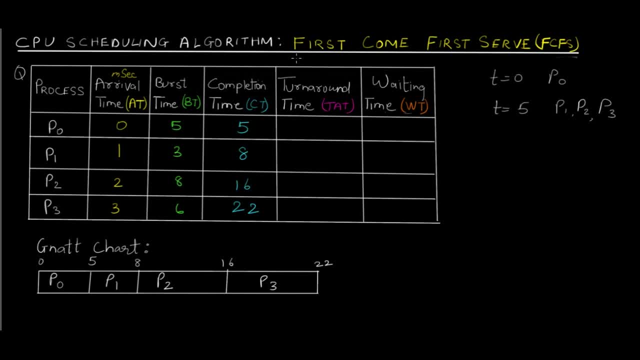 the Gantt chart, the turnaround time. we have a formula for that that is c1. ct, that is completion time minus the arrival time, 80. so we have 5 minus 0, which is 5, 8 minus 1, which is 7, 16 minus 2, that is 14, and 22 minus 3, which is 19. now, if you don't know this formula, 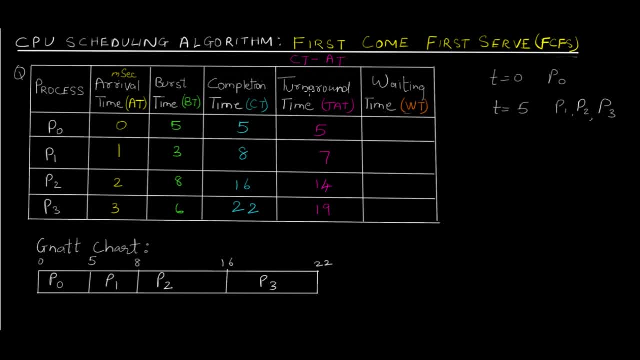 even then you can make out the turnaround time because you know turnaround time is the time spent by a process inside the queue. so just by looking at this process you know that it arrived at 0th second and it got completed at 5th second. so the total time spent inside 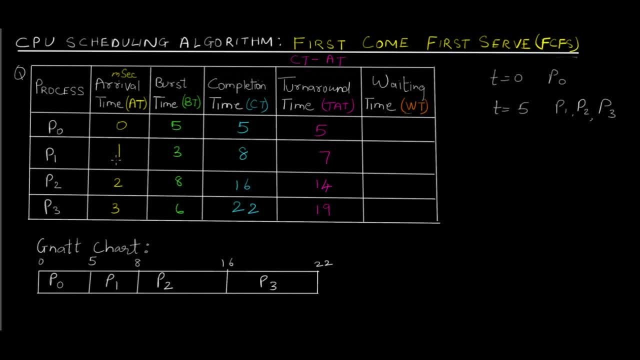 the queue is from 0 to 5. that is equal to 5 for p1. you know that it arrived at 1 second, but it completed at 8 seconds. so 8 minus 1 is going to be 7. so 7 seconds is the time. 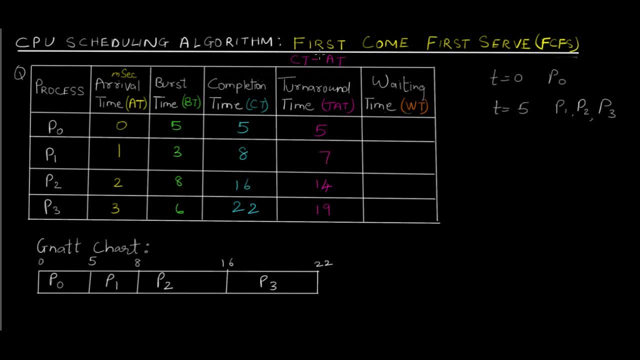 it spent inside the queue. similarly for p2 and p3 also, so you don't really need to learn this formula now. for waiting time, we again have the formula that is turnaround time minus burst time. so 5 minus 5 is going to be 0, 7 minus 3 is going to be 4. 14 minus 8 is going. 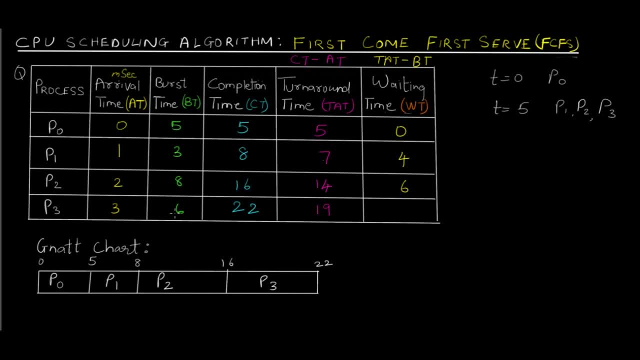 to be 6, and 19 minus 6 is going to be 13. another way to calculate waiting time is: you can see when it came. so, for example, p0 came in at 0 and p2 came in at 0 and p3 came in at 0. 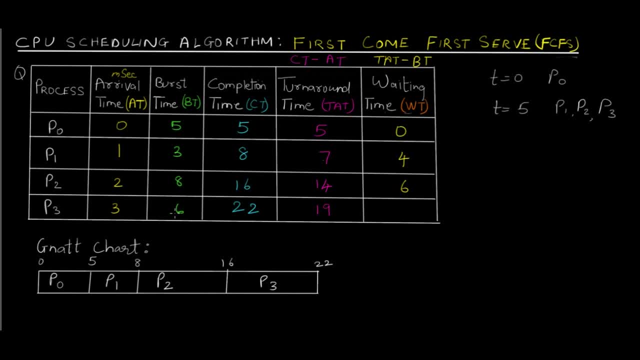 time and as soon as it came the processor started processing it, so it didn't have to wait right. so you can see the waiting time is going to be 0 for p1. you can see that it came at arrival time at 1 second, but it actually started its process, or cpu actually started. 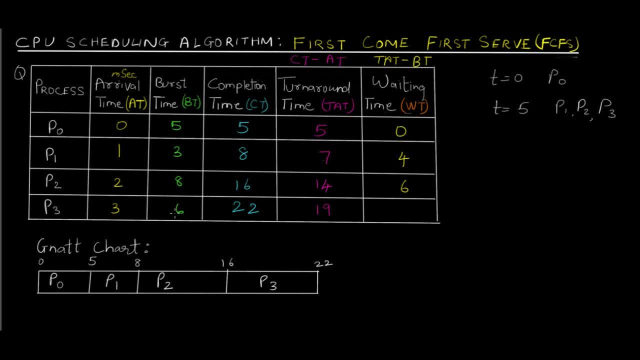 processing p1 at 5th second. so 5 minus 1 is equal to 4. so this is how you get waiting time for p2. also, you can see that it arrived at time 2, but it actually started at 8 second. that is, cpu actually started processing p2 at 8 seconds. so 8 minus 2 is going to be 6. 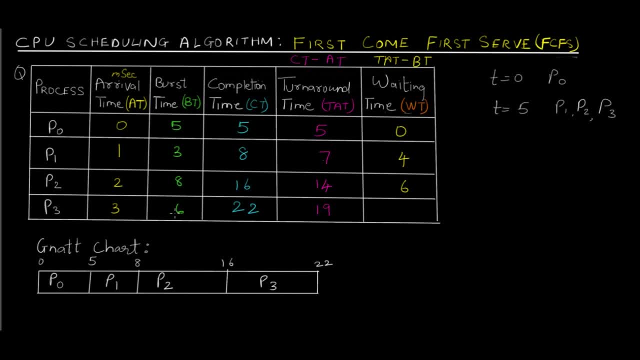 and lastly, for p3 came in at 3rd second but it actually started processing at 16 second. so 16 minus 3 is again going to be 30. so you can directly make out waiting time from this and you don't really need to buy hard this formula. so now we have all the individual values. so lastly, in the 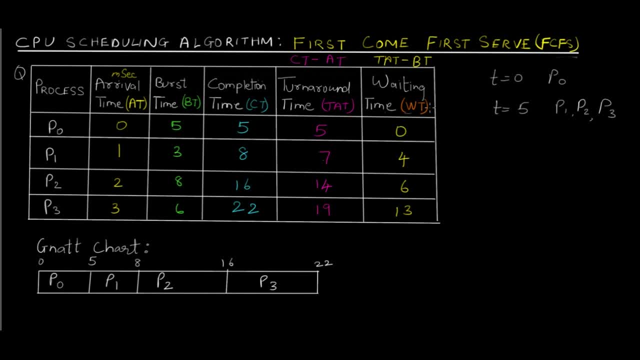 question. we can actually find out the total turnaround time. so we have total tat, which is going to be the sum of these turnaround times, so 5 plus 7, plus 14 plus 19, which is going to be 45 milliseconds. and we can also calculate average turnaround time, so 45 milliseconds. 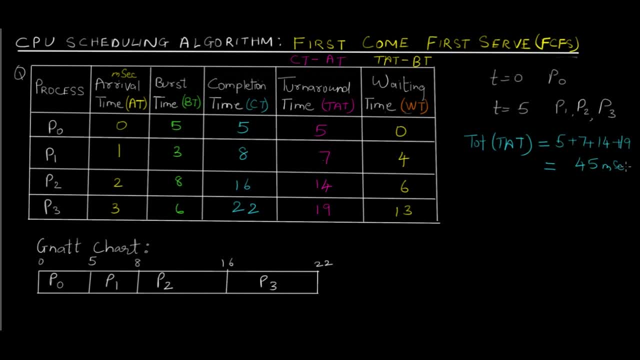 per second and we can also calculate average turnaround time and we can also calculate time which is going to be total TAT, that is, total turnaround time divided by the number of processes, that is, 4, which is going to be 45, divided by 4, which is: